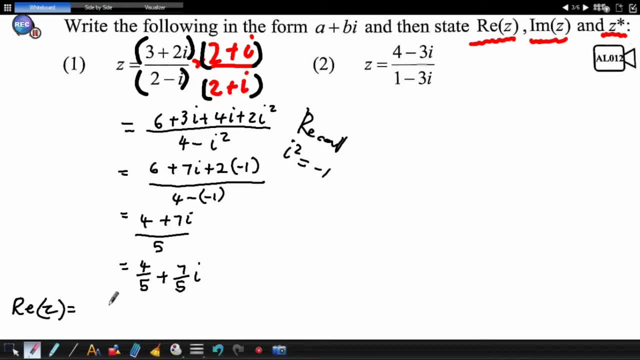 its real part will be four over five. okay, then we have its imaginary part. now its imaginary part will be of: z will be seven over five, and then we'll have now its conjugate, and its conjugate will be four over five minus seven over five i. i hope it was quite clear for. 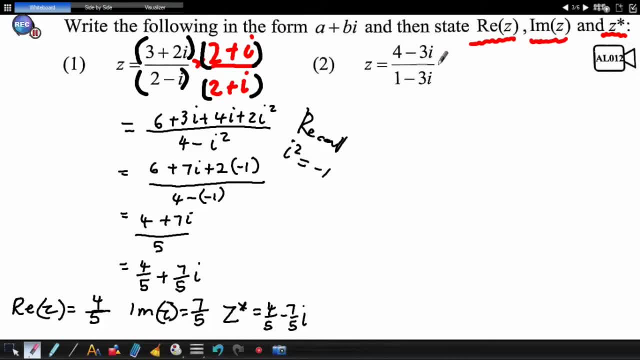 you. let's look at this question, this question again. we are just going to look at what is. it's the conjugate of the denominator. the conjugate of the denominator will be one plus three i and one plus three i. okay, so if now i then want to, 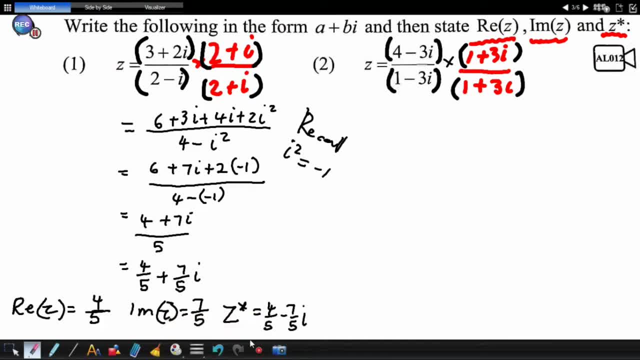 work this out by simplifying. i'm basically going to do the same thing i do. i'm going to do the same thing i do, and i'm going to do the same thing i do and i'm going to in this question. so i will have- i will have four times one, which will just give me four, and then four times three i, which will 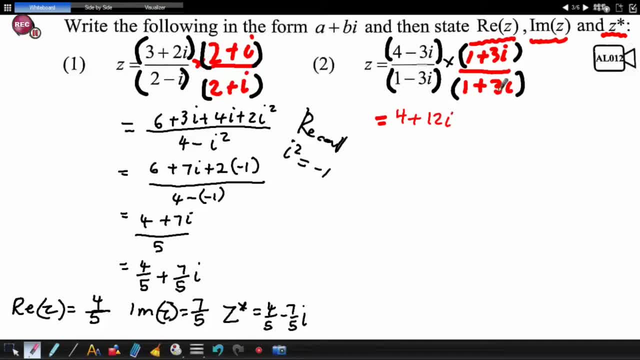 give me 12 i, then three i times one will give me minus three i. and then negative three i times by three i, which will give me negative nine i squared right. and then we at the bottom we're going to have one minus nine i squared. then we can see, guys, a difference of two squares, as you can see there. 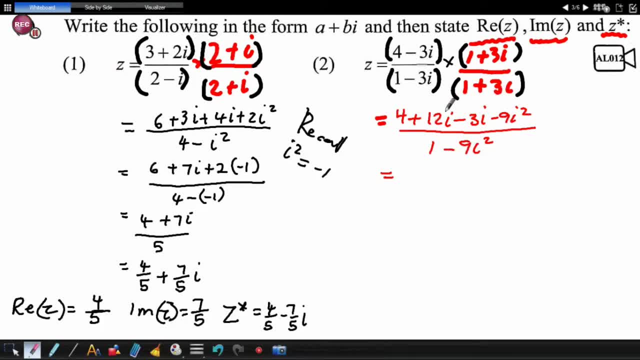 that's why it's so easy to do the denominator. now, all that i'm going to do is collect the like terms. so 12 i minus three, i will give me plus nine i, and then i can see here i can straight away just work this out, guys, if i have. 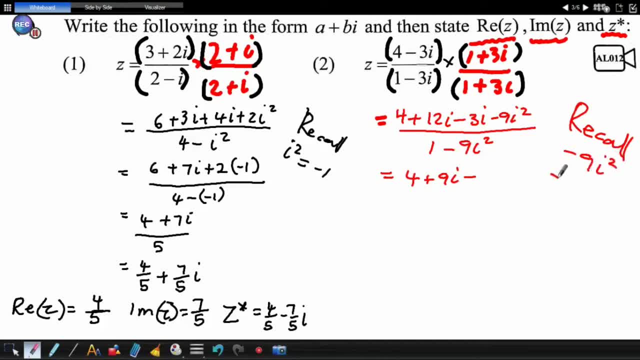 negative nine: i squared. this will give me negative nine. if i substitute one there, it will be positive nine, so let's just go ahead and write positive nine over this. also, again, we have negative nine- i squared. okay, that means it's going to be one plus nine, because we've seen that this negative. 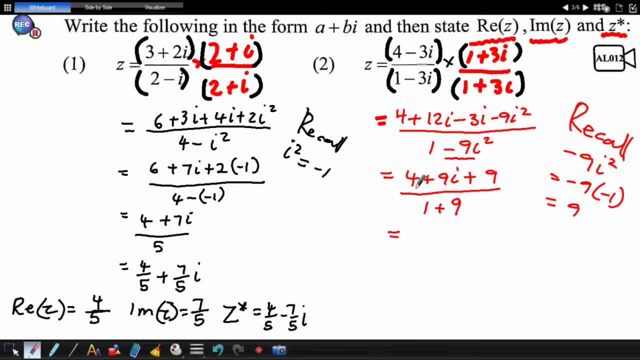 nine i squared is just nine. so the answer then will be four plus nine, which will give you 13 plus nine i squared. so this will give me negative nine i squared. so this will give me negative nine i squared. so this will give me negative nine i over ten. this means that we can write this as a plus b i will be 13 over 10 plus nine over 10 i, meaning we'll have the real part of z, which will be just 13 over 10, we'll have the imaginary part of z, which will be nine over 10, and then we will have its conjugate. 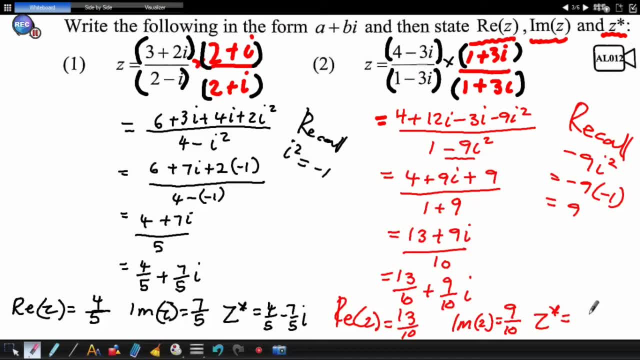 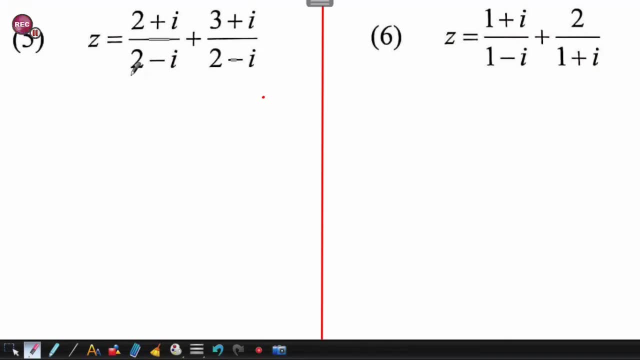 and the conjugate of this complex number will be 13 over 10 minus nine over 10 i. and that's it for this question. we're going to move on. okay, guys, let's look at number five. for number five, we see something: the denominators are the same. that means we are allowed to add the numerators. so 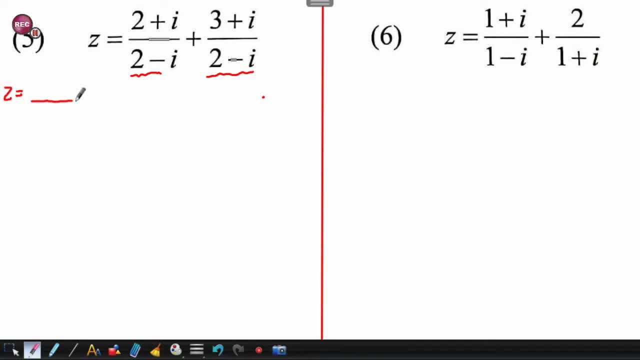 we will have: z is equal to, then the denominator is going to be two minus i, and then at the top we're just going to add: so have five plus two i. okay, another thing that i just have to give you a heads up on. for example, let's say that i had two plus i over, two minus i minus three plus i. 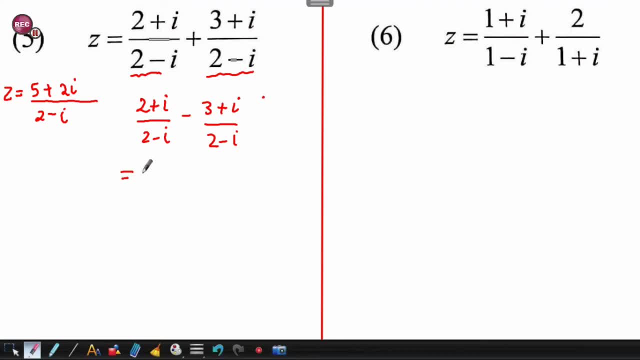 over two minus i. guys, if i had to add that, i would have two plus i and then minus. in brackets i'll have three plus That's just a heads up that you have to take note of, because that negative will distribute the three and then will distribute the I. 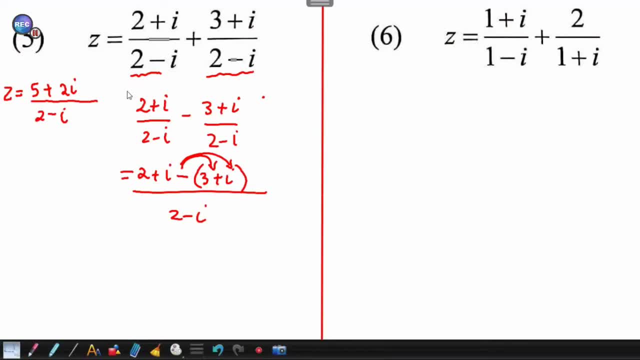 OK, so that's just a by the way. Now, if I want to, because the question then says simplify. So we have to get in that form: A plus B I. So that means I have to introduce the conjugate. So let me introduce a conjugate of the denominator, which is going to be 2 plus I over 2 plus I. 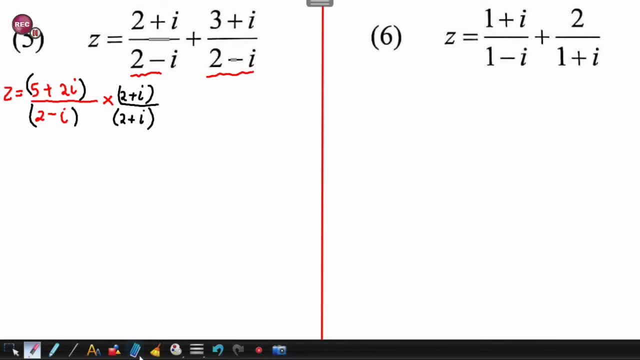 Straight away, introduce my brackets. Then if I simplify this now, I'm going to go ahead and simplify at the bottom. It's quite straightforward: Difference of two squares. So I have 4 minus I squared, And then at the top we'll have 5 times 2, which will give you 2.. 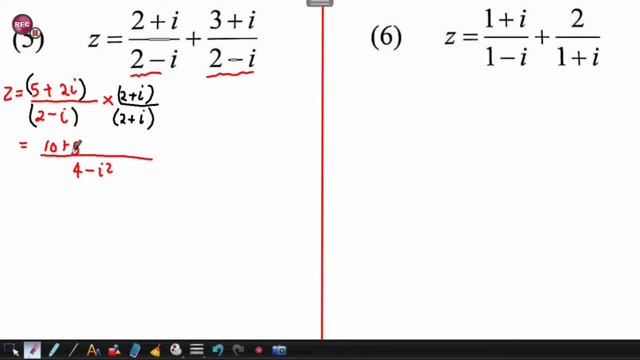 And then 5 times I, which will give you 5I. And then 2I times 2 will give you 4I. And then 2I times I, which will give you 2I. squared Right Now, let's collect the line terms. 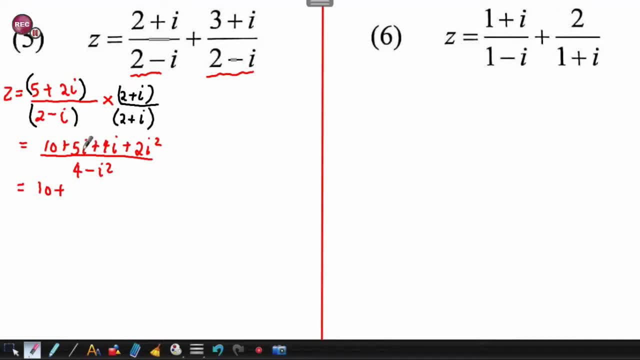 We'll have 10 plus 5I plus 4I will give you 9I. Then, guys, we can recall something that we know: that I squared can be replaced. It's replaced as negative 1.. So we're going to go ahead and just replace it. 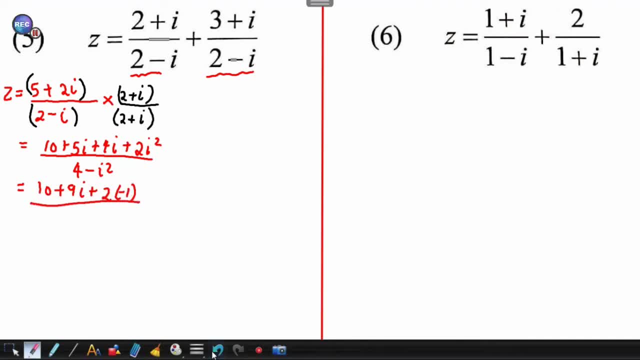 Put a negative 1 there Over, Okay, Say over Over 4. And that I squared is going to be negative 1.. So negative 1 times negative will give you a positive, I A positive 1, sorry, Then the answer now is: 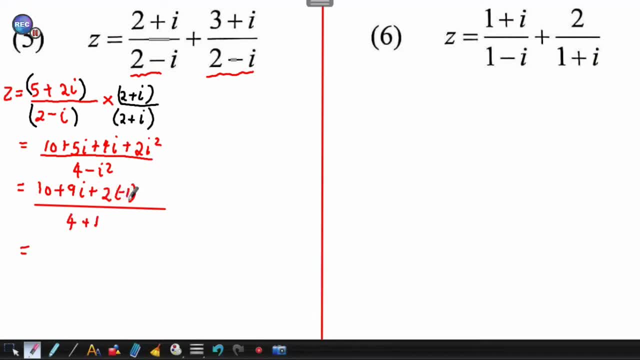 If you see, here you have 2 times negative 1, which is negative 2.. So if you say 10 minus 2,, which will give you 8 plus 9I over 5.. Now this can be written as 8 over 5 plus 9 over 5I. 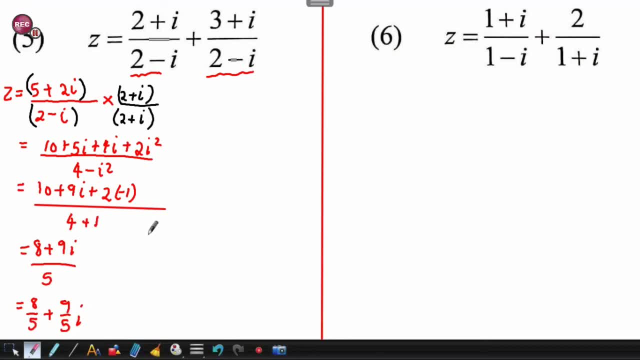 So that means we'll have its conjugate Right. So we'll have its conjugate Right Minus 8 over 5, minus 9 over 5I. Then we'll have the real part of Z, which is 8 over 5.. 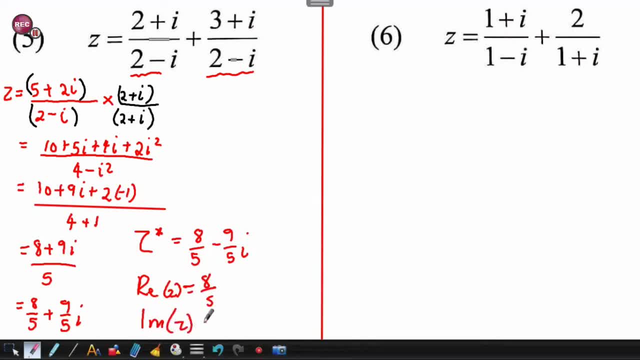 And then the imaginary part of Z, Not its conjugate, guys, It will be 9 over 5.. Right, Let's move on to number 6.. For number 6, guys, there's different ways you can think about this. 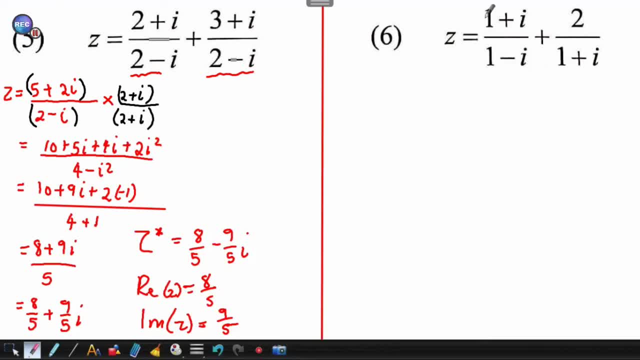 But I'm just going to go ahead and tell you that if we have 2 fractions, we need to add those fractions to simplify before we can do any other thing. And I see that we have 1 minus I and we have 1 plus I. 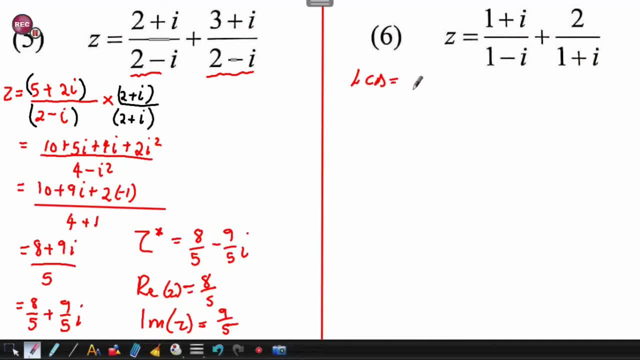 So let's find the lowest common denominator. The lowest common denominator would be 1 minus I and 1 plus I. Okay, So that means for this fraction, I'll have to multiply it by 1 plus I over I. So what do I mean by this? 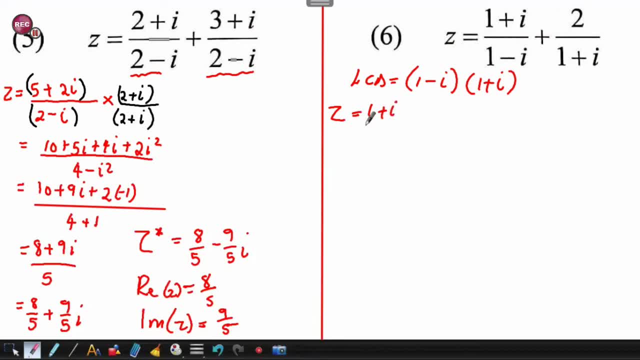 Okay, So I'm going to multiply it by 1 plus I over I. This is what I mean: 1 plus I over 1 minus I For me to have this denominator. this fraction is short of that 1 plus I at the bottom there. 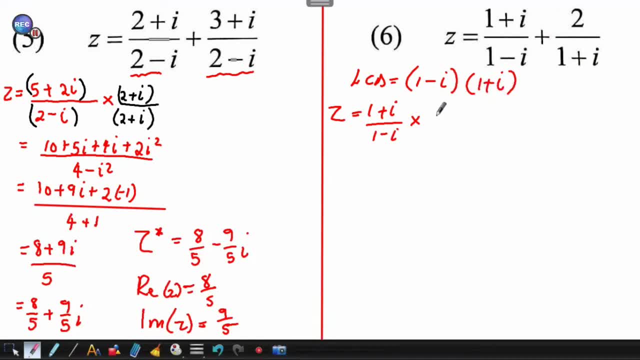 So the denominator is short of 1 plus I. That means I have to multiply 1 plus I over 1 plus I And you would say that's the same as just multiplying with its conjugate. Yes, So 2 over 1 plus I. 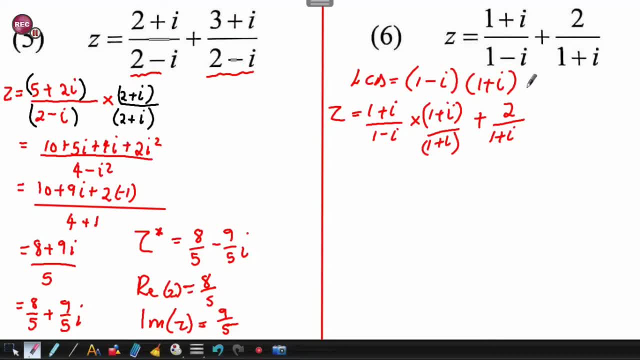 So 1 minus I, over 1 minus I. For me to have this denominator, that means I have to multiply this fraction by 1 minus I, over 1 minus I. Then now let me simplify. If I simplify at the top, guys, the bottom, straight away, it's going to be 1 minus I, squared. 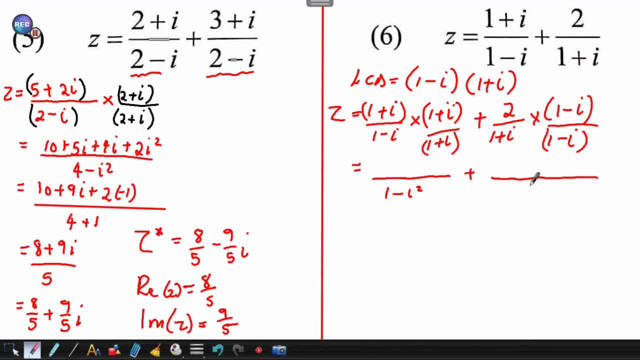 Okay, Also here the bottom- we're going to have 1 minus. I squared- It's quite straightforward- right At the top. there we can see that we have 1.. So let me just go ahead and say this will be 1 plus. 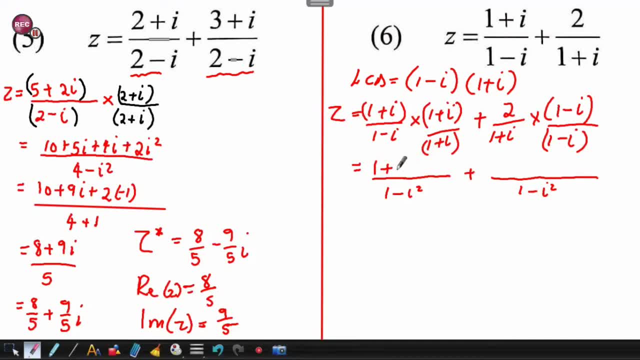 This will be 1 times I, which will just be I, And then I times 1,, which will just be I, And then I times I, which will then be I. squared Right Here at the top. it's quite straightforward. 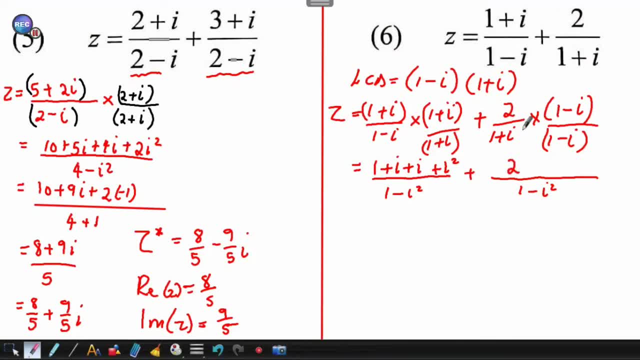 So we'll just have 2 times 1, which will just be 2.. And then 2 times negative- I will just be Minus 2I. Right Things are coming together, guys. Okay, Now we see we have the same denominator. 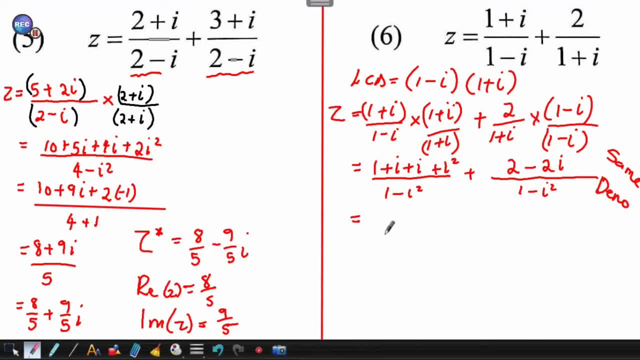 Right, So that means we can add the numerator. Okay, The numerators can be added, because the denominators are the same, So we'll have 1 plus I. Okay, Let me just go ahead and say that is just going to be 2I. 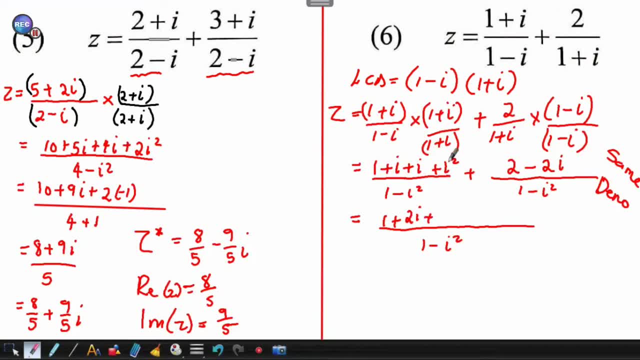 So we'll have 2I plus That. I squared guys. I'm going to go ahead and just write it as negative 1 plus Okay, And then we'll have plus 2 minus 2I. Look at what happens there. 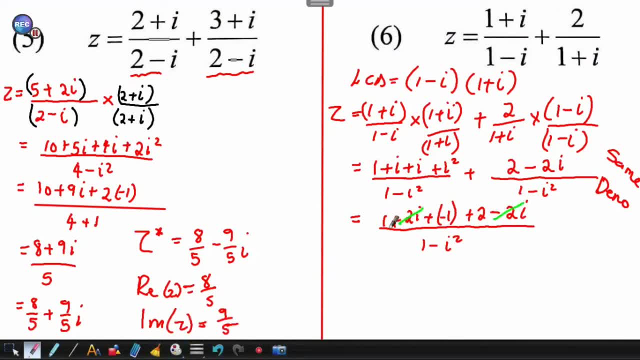 That 2I will cancel this guy, And then you have 1 plus 2,, which will just be 3.. So let's just see, We'll have 1 plus 2,, which will just be 3.. Minus 1,, which will just be 2.. 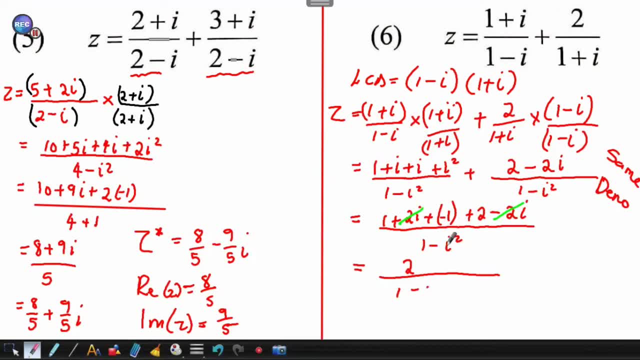 Over 1 minus- Oh, I forgot to substitute here- We'll get negative 1.. So therefore, you have 2 over 2, which the answer is just 1.. We're not done. They asked for what is the real part. 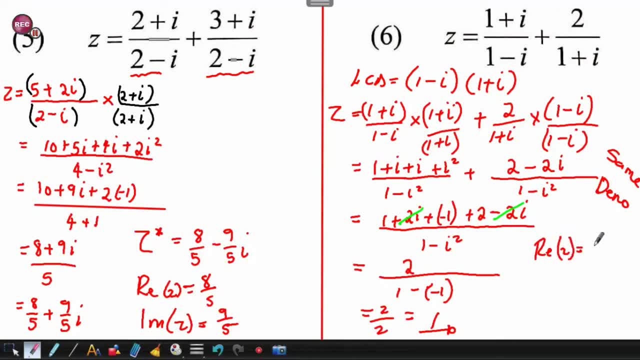 Oh see what I was saying. The real part is 1.. What is the imaginary part? The imaginary part, you'd say: okay, The imaginary part Is 0.. I, sorry, is just 0, because this number, guys, can be written as in the form a plus B, B. 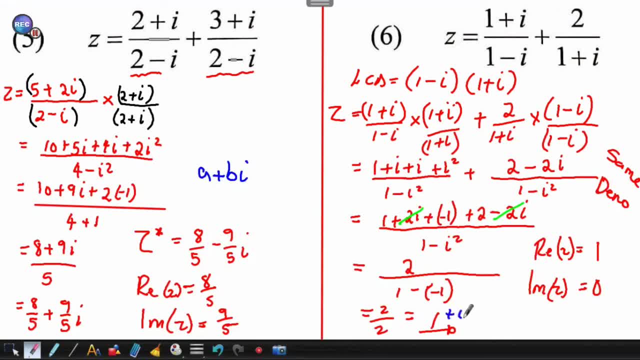 I. then this will just be 1 plus 0.. I that's why we're seeing the imaginary part is 0 and the real part is 1.. Then it's conjugate. Now it's conjugate will be just 1, because if we were to change this, 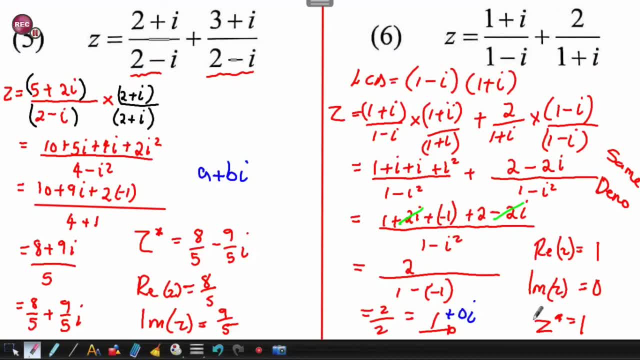 it will be negative 0, I, which will just be 0. So hence that's conjugate is also 1.. This was a nice question. That was nicely challenging.